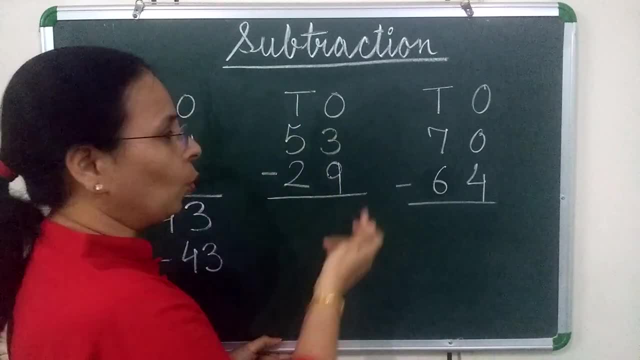 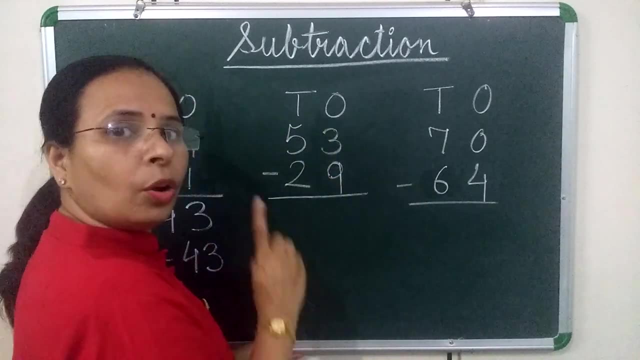 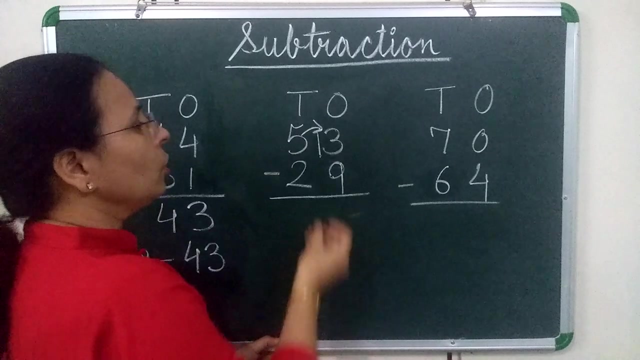 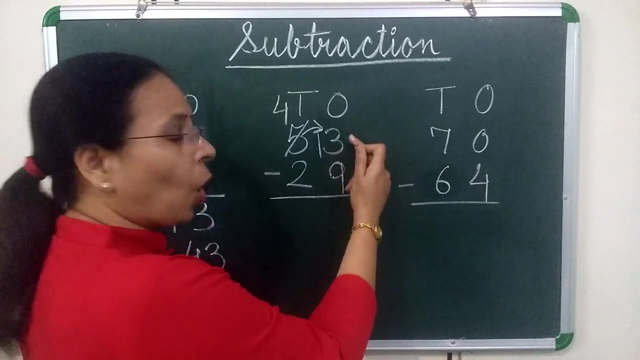 And 3 is greater than 9.. No, it is less than 9.. So 3 will borrow 1 from 5 and it becomes 13.. 5 has given 1, so 5 becomes 4.. Now we will subtract 5 from 13.. 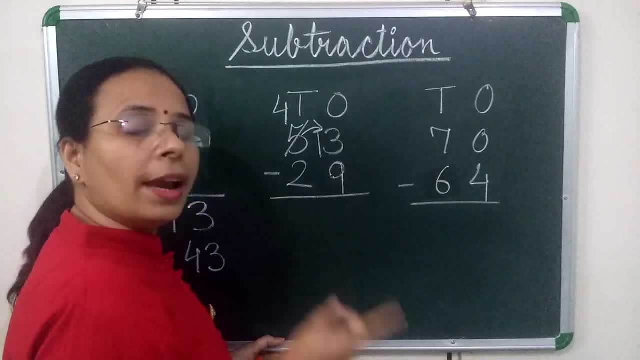 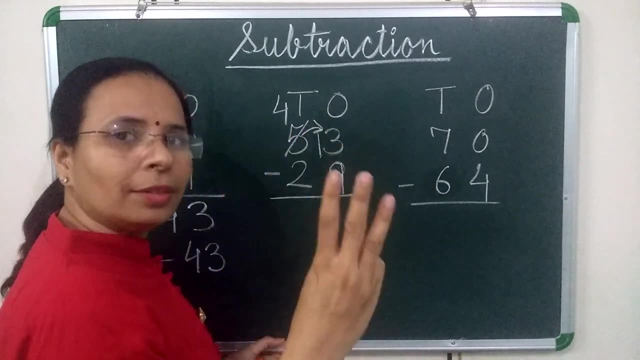 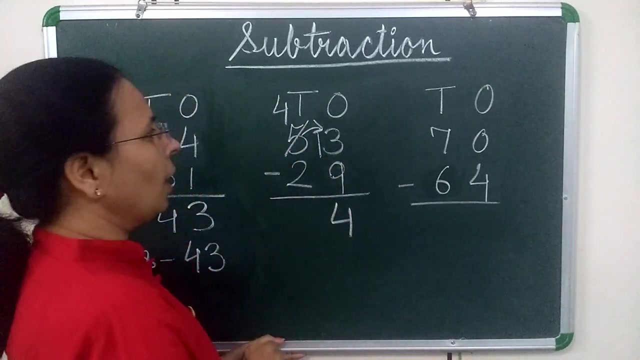 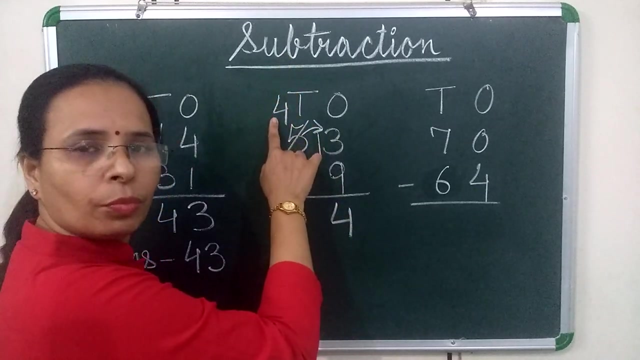 Now we will start counting after 9.. And till 13.. What comes after 9?? 10,, 11,, 12,, 13.. So how many fingers are out? 4. We will write 4.. Now, here we have to subtract, at 10th place, 2 from 4.. 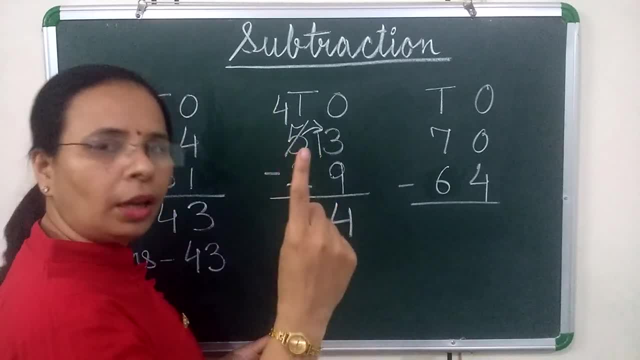 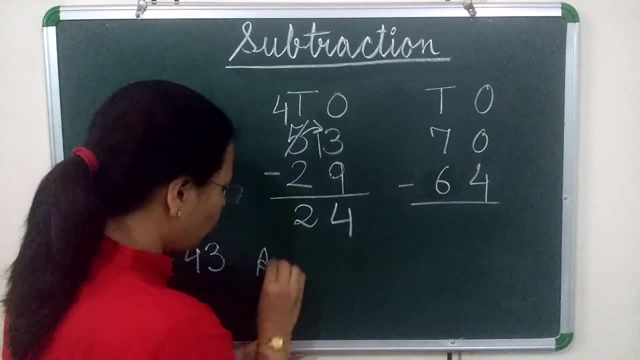 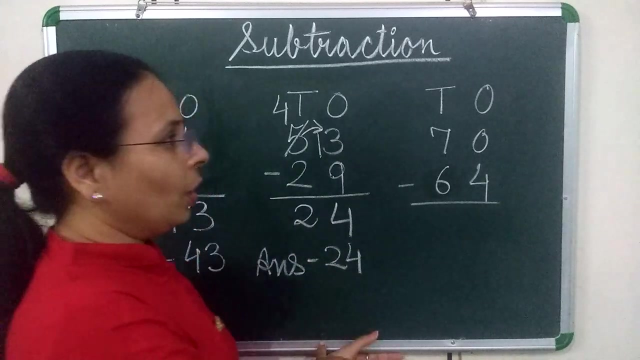 So what comes after 2?, 3,, 4.. So how many fingers are out? 2. We will write 2.. Children 24 is our answer. Now we will move to third question. Now, here, at one's place, first number is 0,. second number is 4.. 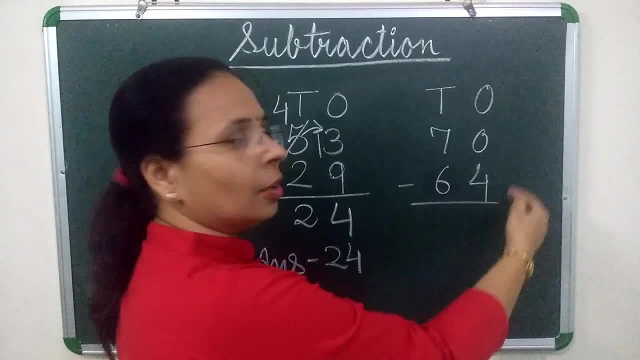 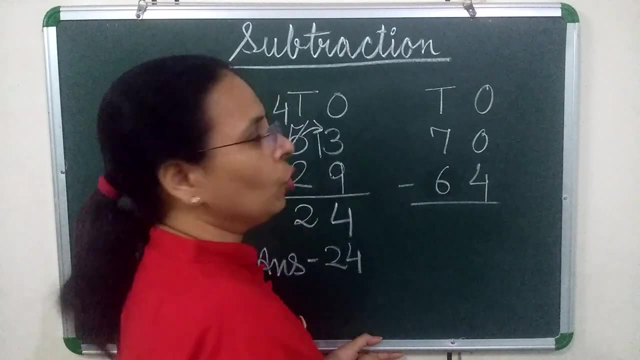 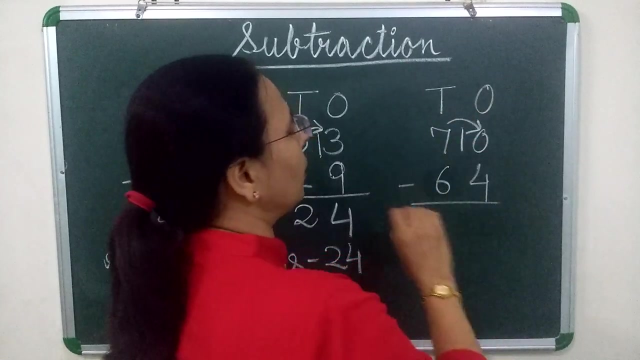 You remember from where we have to start? From one's place And one's place. first number is 0 and second number is 4.. What we will do? We borrow 1 from 7.. Now 0 becomes 10 and 7 becomes 6.. 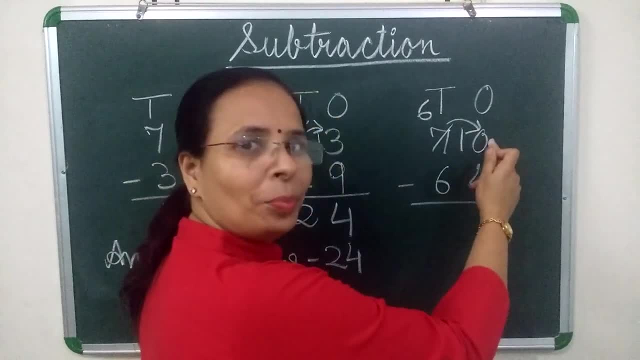 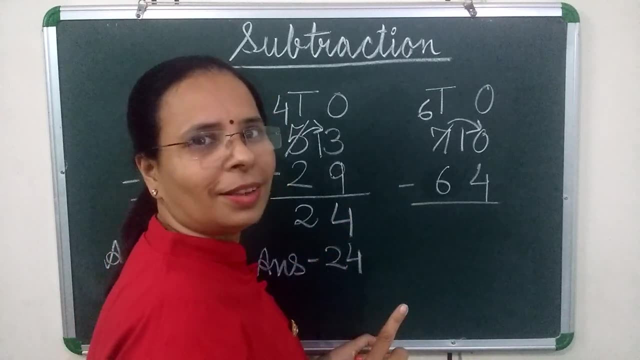 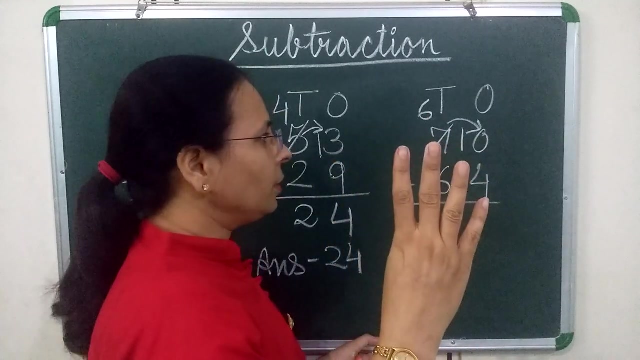 Now we will subtract 4 from 10. And we will start counting after 4 up till 10.. So what comes after 4?? 5, 6, 7, 7, 8, 9, 10. So how many fingers are there? 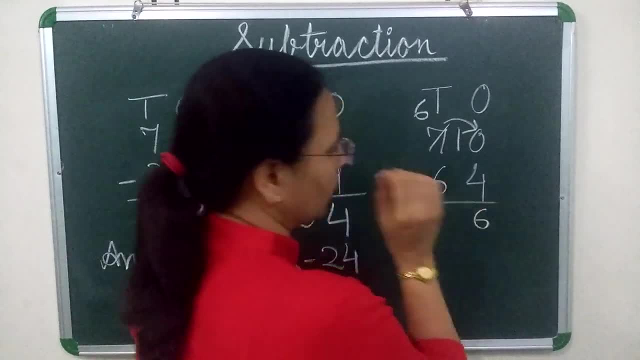 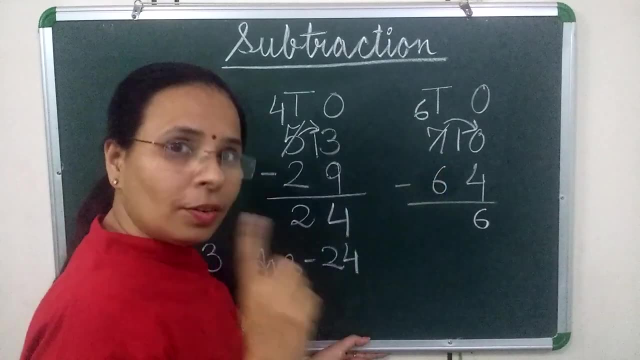 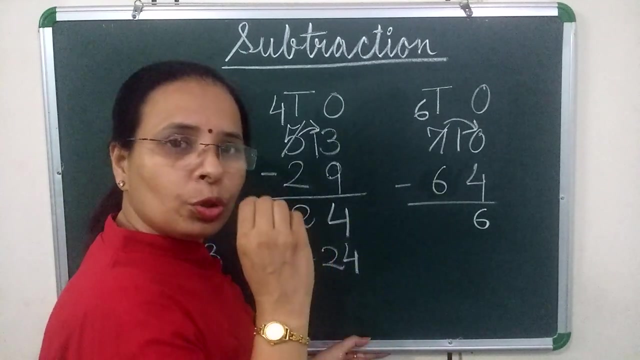 6. So we will write 6.. Now children see, at 10th place we have to subtract 6 from 6.. Always remember same number. when we have to subtract same number, answer always be 0.. So we will write here 0..